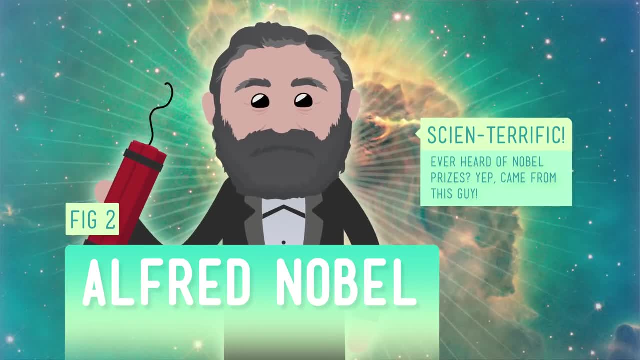 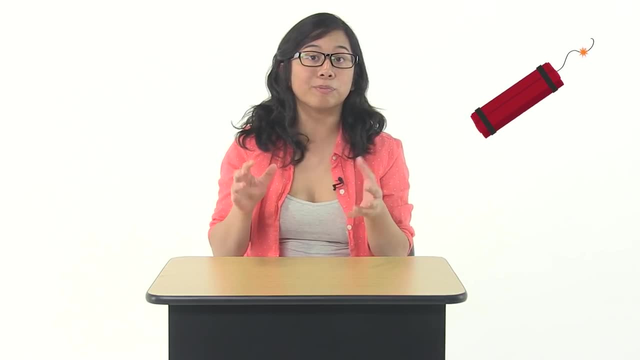 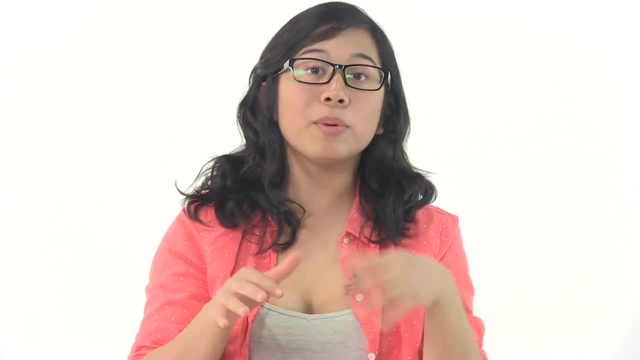 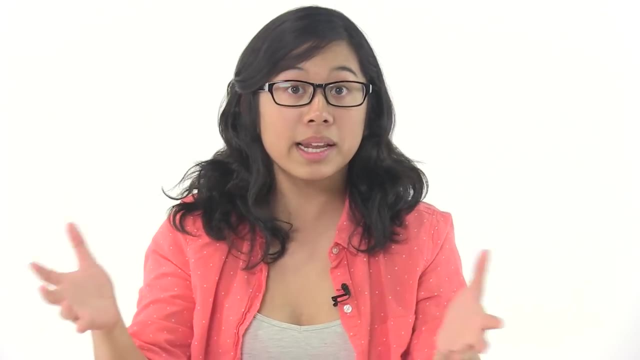 they just couldn't wind up making stuff up to do their jobs needed an explosive that was safer to use. So before he started on that problem, Nobel did research to see what explosives already existed, which ones worked well and which ones didn't. This takes us. 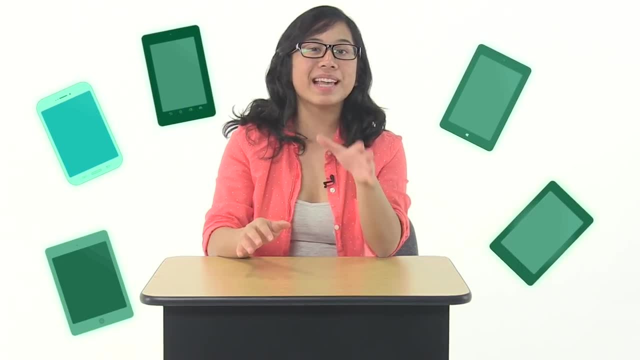 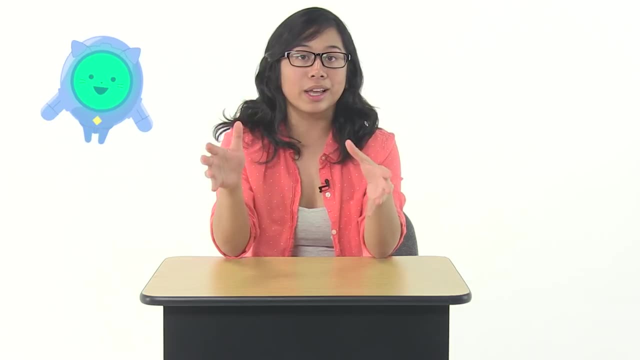 to Step 3. Develop a solution After your research is done. this is where you say exactly how you think you can solve the problem, and once you've thought of a good solution, you have to figure out how it will actually work and what it will look like. So you have to design your solution. 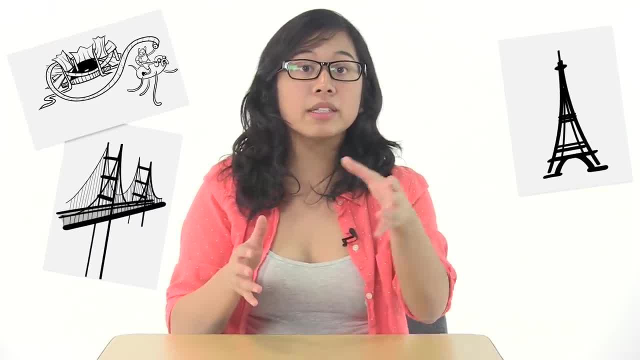 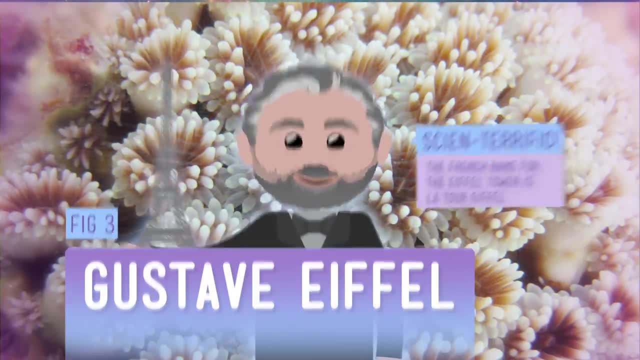 This is where you get to draw out their ideas, like buildings and bridges and towers, to show what they'll look like when they're done. Gustave Eiffel designed the famous Eiffel Tower in France and he definitely showed up on day one of construction knowing exactly what it was going to look like. 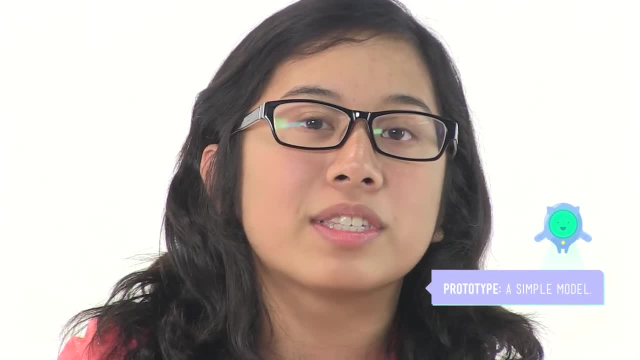 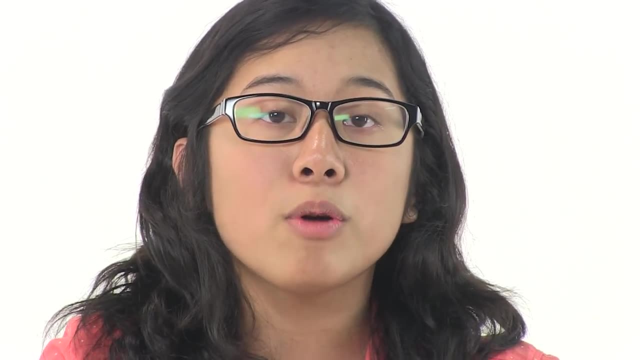 On to step five: build a prototype. A prototype is just a simple model that lets you test out your design. It can be as big as the real thing's going to be, or it can be a smaller version. You just need to have a prototype so you can test it. 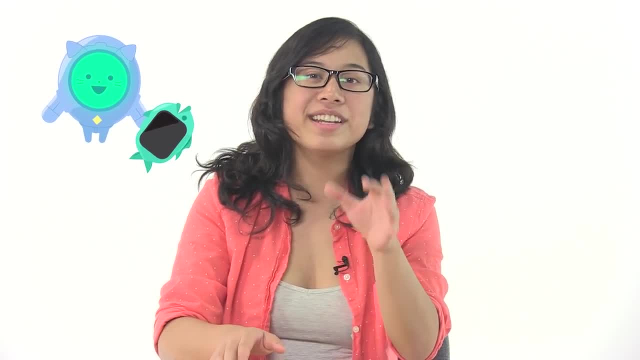 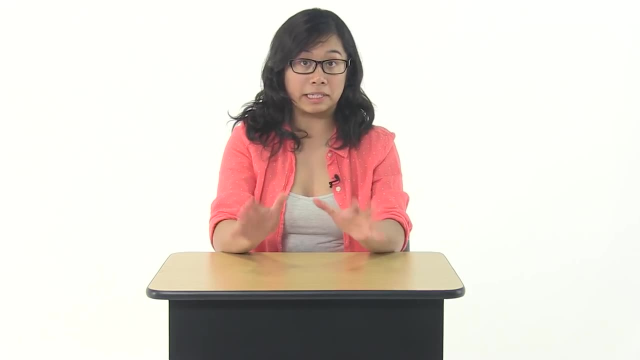 This may be the most important step in the whole process. Engineers need to test their design to see if it works like they want it to. So say, if your building's a big tower, does it stand up? Does it stay standing up? If you're designing something with moving parts, does it work the way you want? 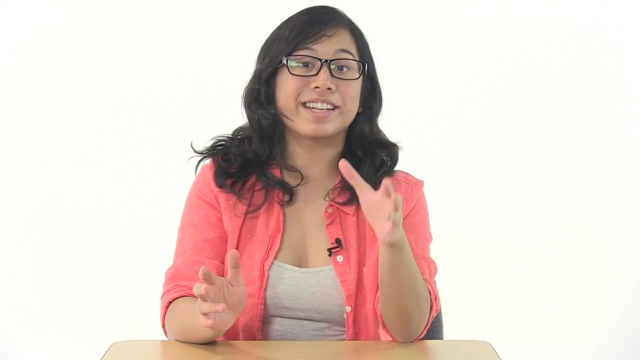 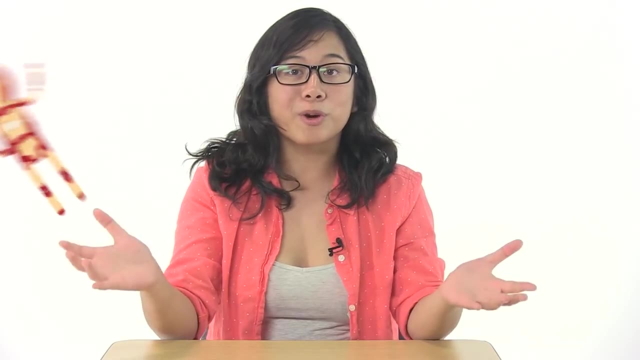 Now take it from me, my future engineers. you might have a great idea, a really terrific solution to a really big problem, but when you get to this step, your prototype probably won't work exactly the way you want, At least not on the first try. 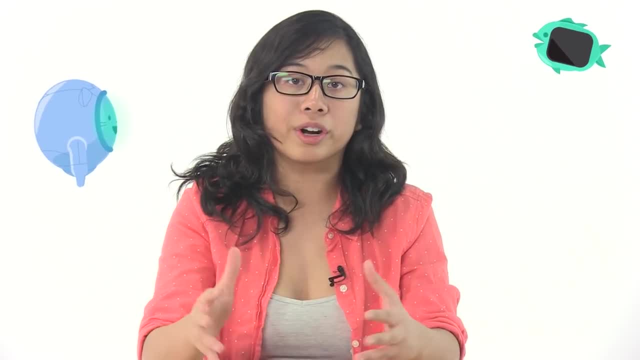 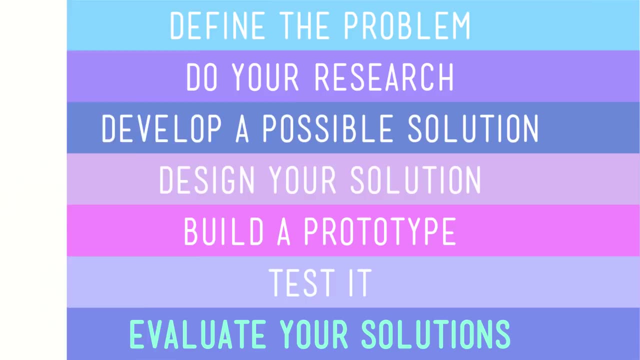 Most engineers test their prototypes over and over and over. That's why a lot of time and brainpower goes into the very last step: evaluating your solutions. Evaluating just means asking yourself whether things are working the way you want, or why they are or aren't.